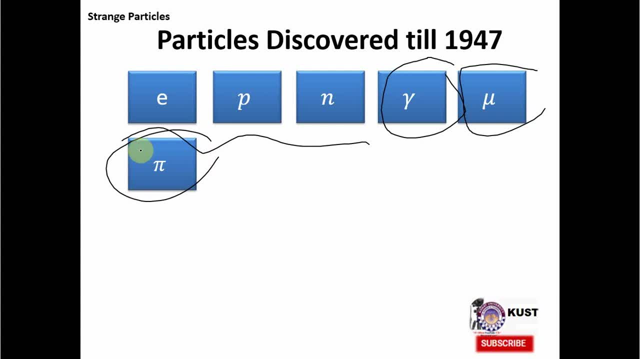 Which we call mesons, because these are the middle weights, And then one another particle we call a neutrino, which is needed in the explanation of the beta decay, where the law of conservation of energy is restored. if we consider that a neutrino is there, 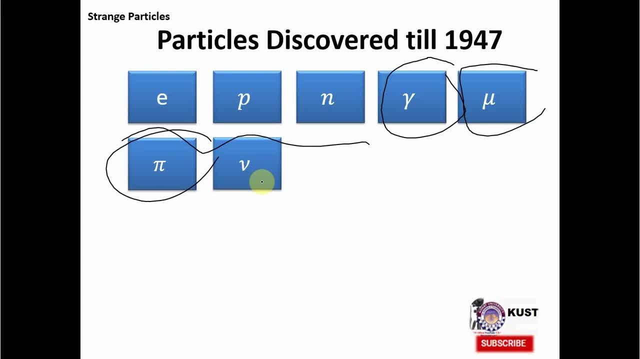 Neutrino is slightly a mysterious particle, but in 1947 it was well understood. So these are the six particles known at that time And there were two theories, Two big theories. One of them was quantum mechanics, which was very much involved into the particle physics. 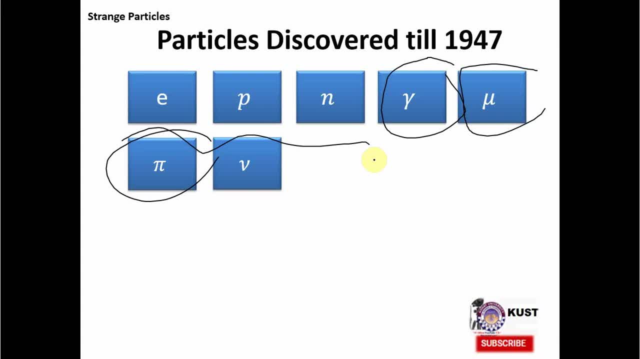 And the second one was Einstein's special theory of relativity. And from the requirements of special theory of relativity we knew that we have to have antiparticles, That is, every particle has its own antiparticle. And if I list them, you see here the electron has an antiparticle. 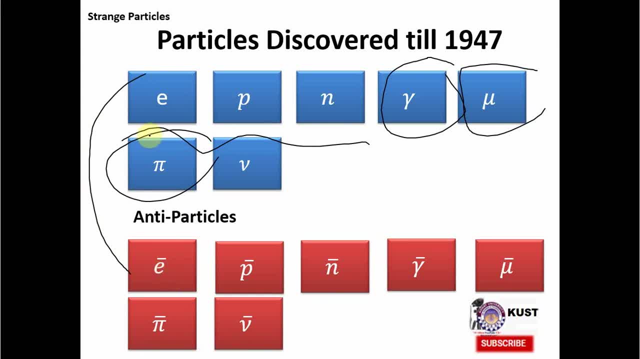 We call it a positron, And positron is electron, similar to the electron And in all respects, only not in the charge, where it has a positive charge. Similar is the case with a proton: It has antiproton, But in case of the neutron, because it's charge-less, there is no charge. 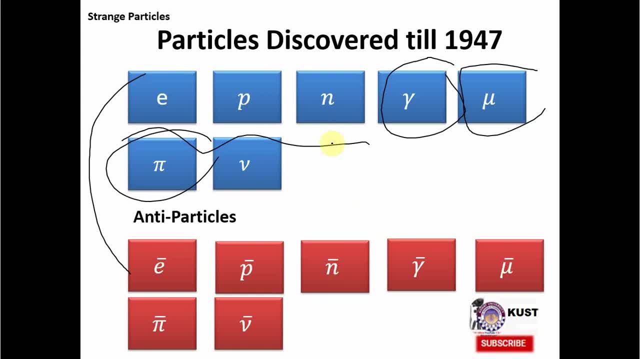 But there are other quantum numbers where antineutron is different from neutron. More interestingly, photon is actually its own antiparticle, because there is no property which differentiates between photon and antiparticle. And then we have antiparticles too. 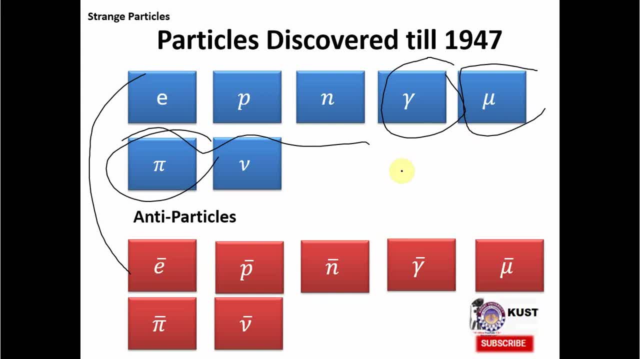 All these known particles. This is another question, that why at the moment we have more particles than antiparticles, which is not still we don't know the answer to this question yet. But at that time, in 1947, we had only 14 fundamental particles. 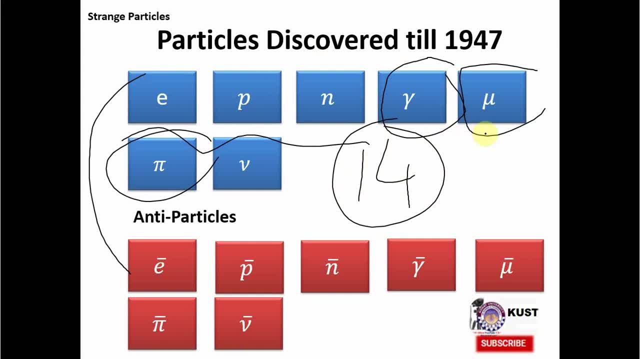 to explain not only the structure of the atom but also the interactions known at that time. Mind you, these particles were at that time considered fundamental, But later on we found that some of them are not. For example, proton has a structure, neutron has a structure. 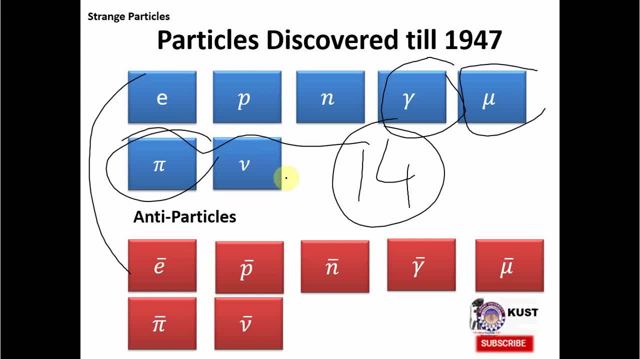 although electron and neutrino, they are still considered to be fundamental particles. By fundamental we mean that they have no further structure. But these 14 particles make a picture very simple, And this state of comfort actually did not last very long, because we had few particles that could explain the structure of the matter and the interactions. 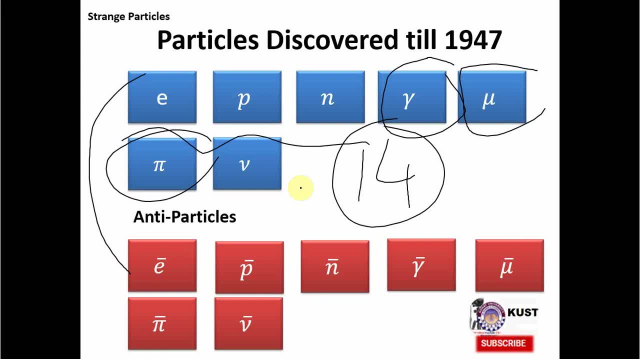 Very nice picture, very comfortable, Very comfortable picture. But, as you know, in physics we always have a situation where we think that everything is complete, We have a complete description for everything, But then some discovery actually destroys this state of comfort. 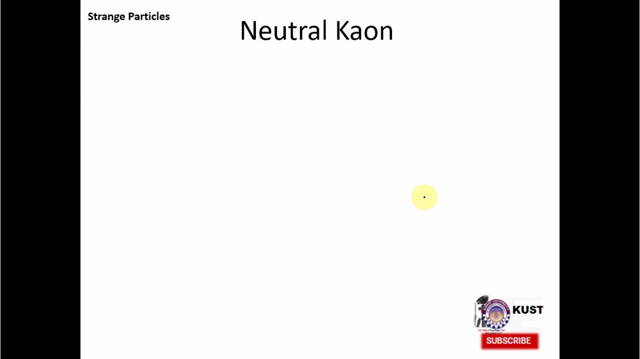 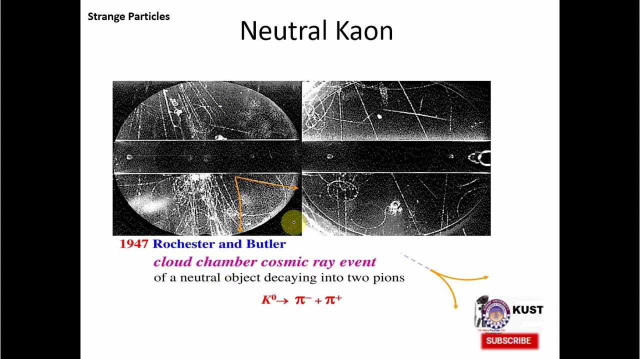 And at that time, the discovery which destroyed this state of comfort was a discovery of another particle called a neutral kaon. In the December of 1947, two scientists, Roche and Butler, actually were doing experiments with a cloud chamber on cosmic rays. 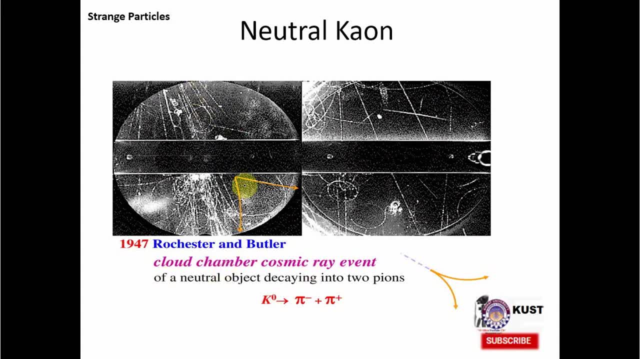 Here you see that the shower of cosmic rays coming down, And they found out that this V-shape where they have two pions, that is a kaon going into the two pions, And these two pions were used to discover that there is another particle called kaon. 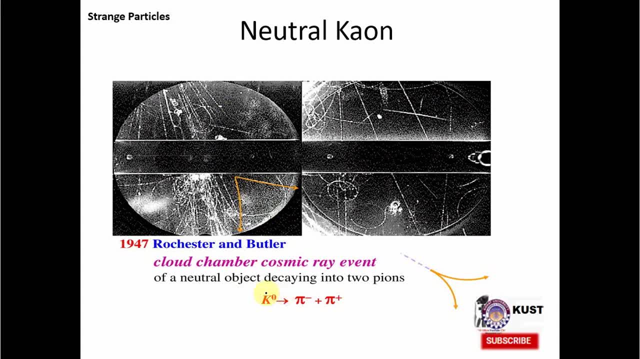 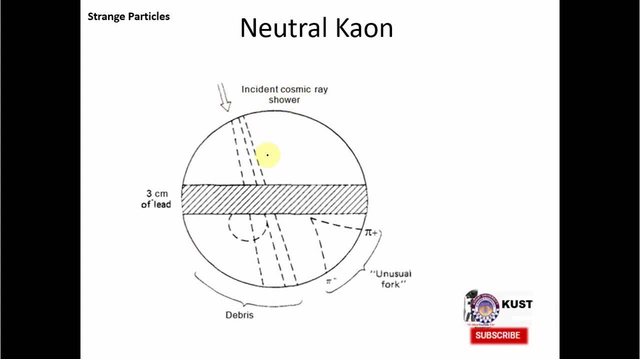 And this particle was put into the family of mesons. If we go into the schematics you can see a better picture where you see that incident: cosmic rays shower coming down from the heavens, from the skies, And then it is split into two particles. this kaon. 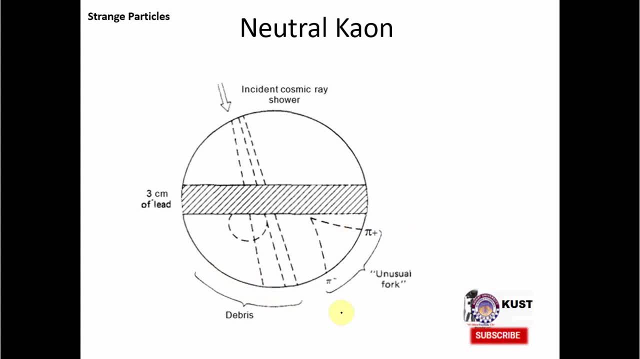 pi plus and pi minus, And these are actually the debris And these two particles. we already know about them, but we discovered a neutral kaon. Why it was not welcomed? Because you don't need it for the explanation of the structure of the atom. 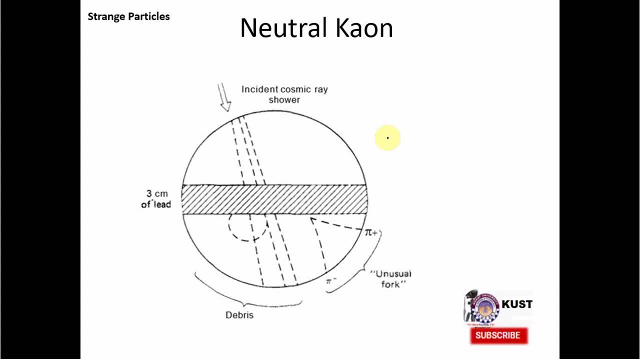 You don't need it into the mediation of any force. So it was actually not needed, But it is there, it was there, it was found. so picture was disturbed And we have to find place for it, place for the neutral kaon, where to put it. 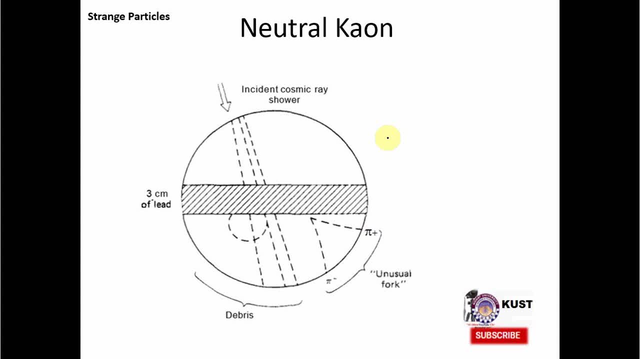 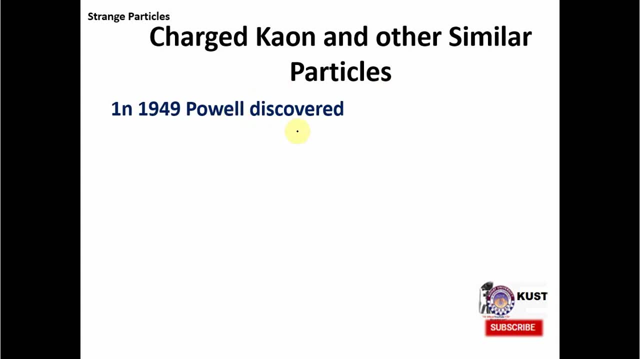 But the story went on getting complicated by discovery of other new particles, For example charged kaons and other similar particles. In 1947, Powell and his colleagues discovered that there is actually another kaon which decays, which is a charged kaon. 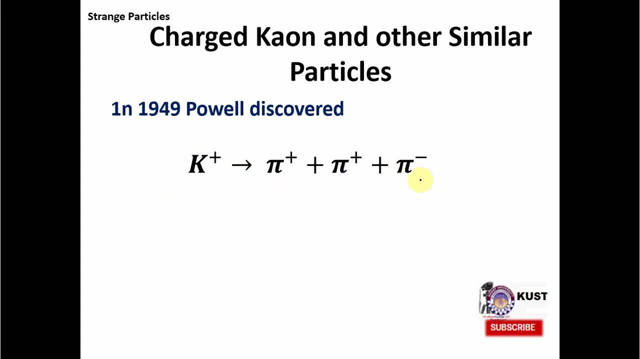 which decays into three pions. So we got the list extended from 14 to 16.. But this was not the end of the story And we discovered even further mesons And the number was going up and up. It came into. hundreds of particles were discovered. 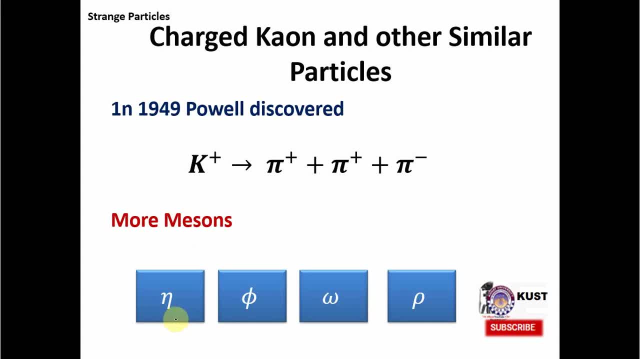 Hundreds of mesons were discovered, And these are a few of the names, for example, given to them: Etos, phis, omegas and ros, and so on and so on. But things were not that worse at that time. 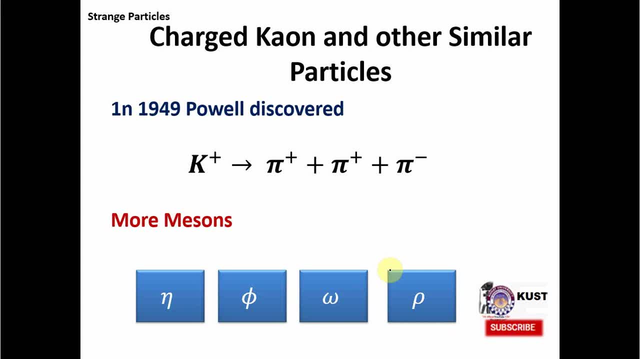 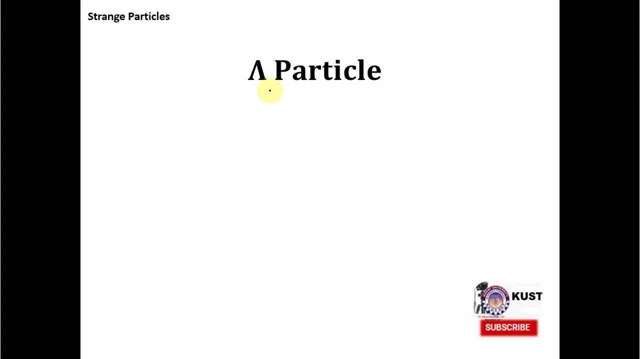 We have few mesons into the list- and scientists, physicists, were trying to understand their properties and trying to put them into right places. And this story was even further worsened by the discovery of another particle called lambda particle. This lambda particle was really a strange particle, because this particle decayed. 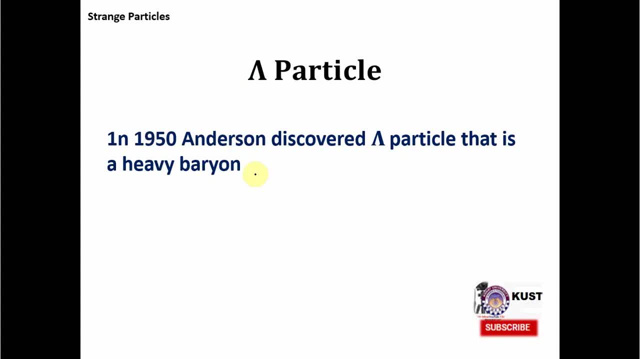 Before that, in 1950, Anderson discovered a lambda particle And it did not belong to the meson's family. It was very heavy and that belonged to the baryon's family, which baryon means heavy particles. So this lambda was decaying into the proton and into the pion. 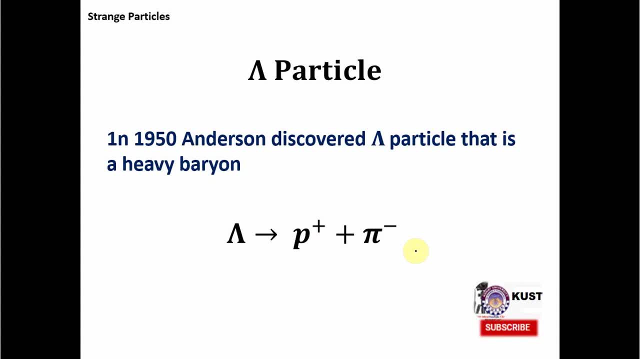 And now, before going into further details of the lambda particle, I want to throw a law here which is called a conservation of baryon number. So we need to understand what is baryon number. So, in order to understand the baryon number, 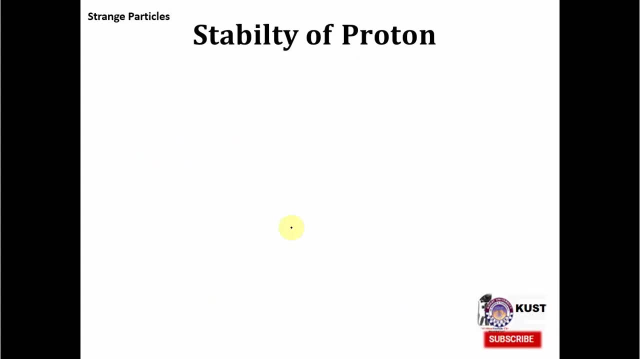 let's go into a slightly different thing, which is called a stability of proton. What do we mean by stability of proton? We know that the atom, or ourselves- we are made up of atoms are stable, And the nucleus of the atom is made of protons, which means proton is stable. 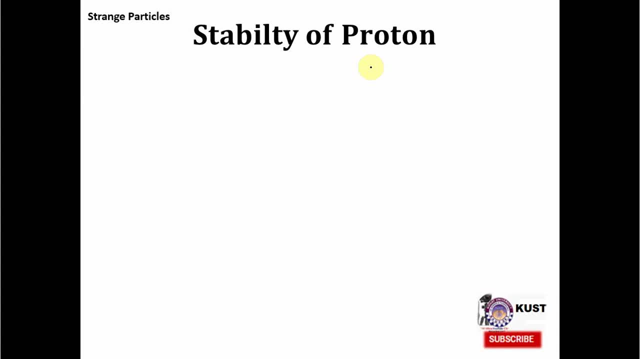 Proton does not decay into other particles. But if you look at this reaction here, this proton actually is allowed to decay into positron, into the gamma rays, And this reaction has no problems, at least in 1947.. All the known laws of conservation, for example. 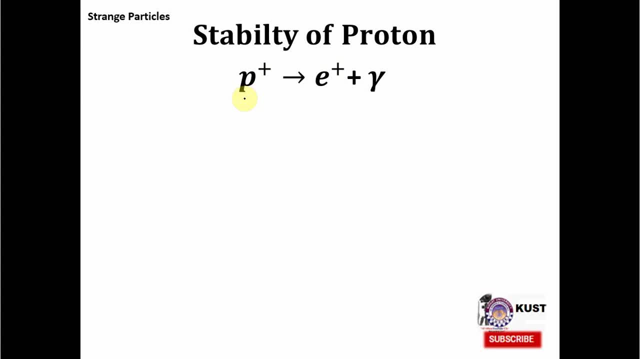 law of conservation of charge is not violated here. Law of conservation of energy is not violated here, Although the law of conservation of electron number is violated here. but that was not known at that time. Now there is a rule of thumb from the Richard Feynman. 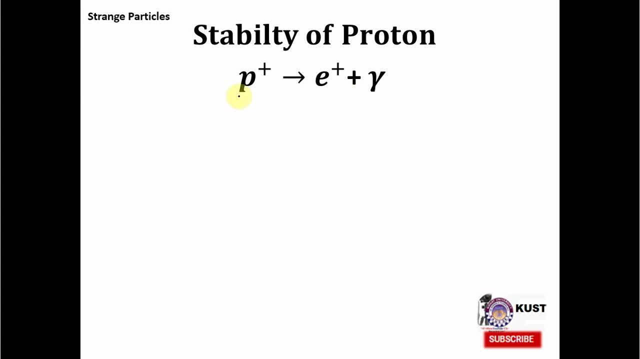 who says that if something is not violated, if some process is not violated by any natural law- law of nature- then it is mandatory that it has to happen Now. surely we don't allow this to happen, otherwise we won't exist ourselves. 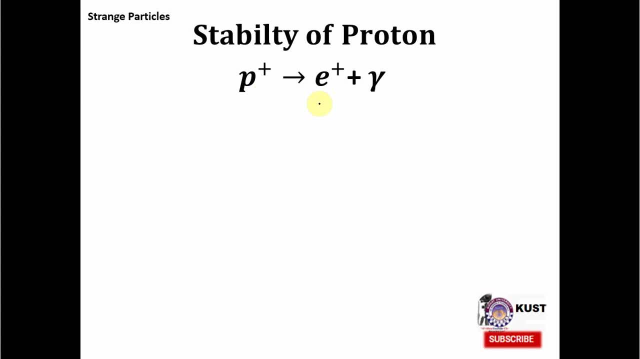 So we need to discover a law which is violated here, And people discovered the law of conservation of baryon number. So in order to put this law into here, we first have to assign baryon number to every particle. So let's assign. 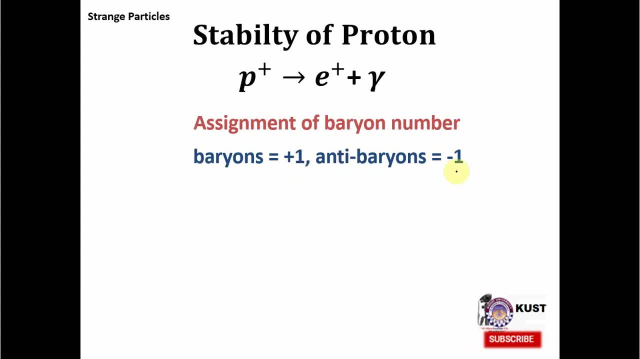 positive one to the baryons and negative one to the anti-baryons and to the rest of the particles. baryon number zero. Now, this assignment is completely arbitrary, But well, this actually helps. You can say that baryons are minus ones and anti-baryons are plus ones. 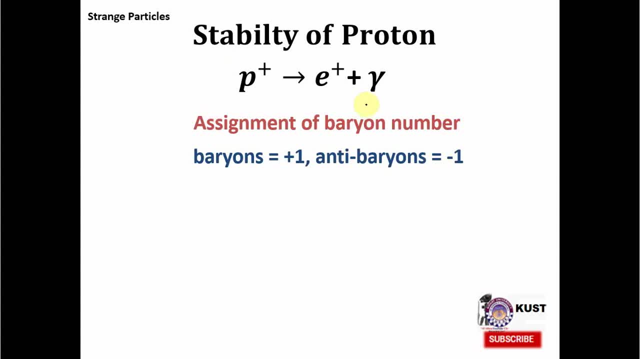 but it doesn't matter At the end. baryon number is not conserved here. If you look at here in light of this new conservation law and baryon numbers, you find out that the proton has a baryon number one. 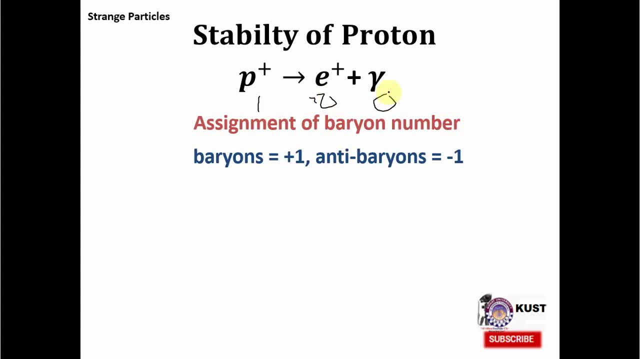 but here these two particles have baryon number zero, So it means that baryon number is violated here and we cannot allow this to happen. So this new law of conservation of baryon number is discovered here, And if you use this law and go to the neutron beta decay. 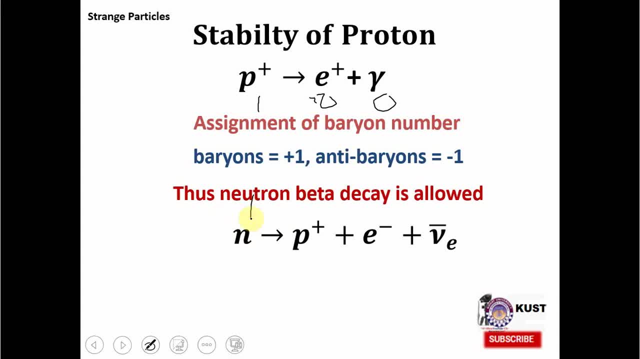 you see that this is allowed because here the baryon number one one, and this is zero and zero. So now, this law, this decay, this process is allowed because of the law of conservation of baryon number, because it's not violated. 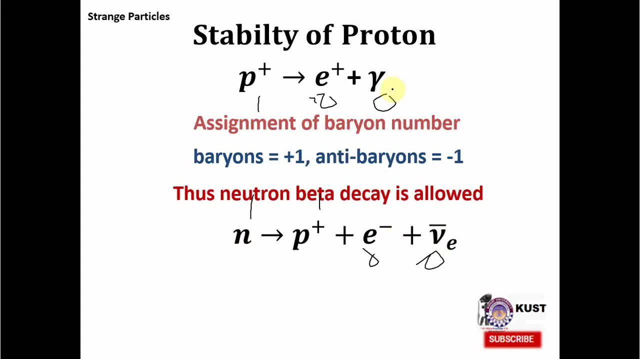 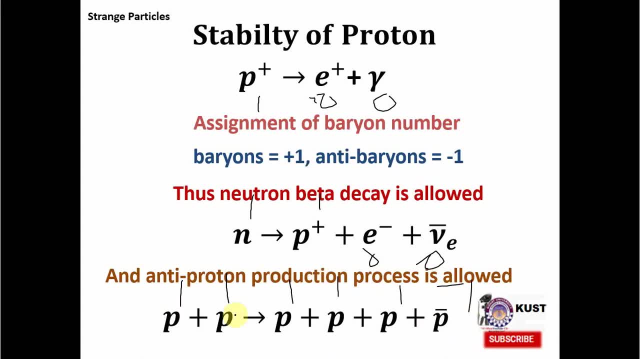 So, since baryon number is conserved, so we actually have the anti-protons produced from the interaction of two protons. and this is a very usual process, done everywhere, For example into the CERN, into the laboratories. people discover so many particles by colliding two protons. 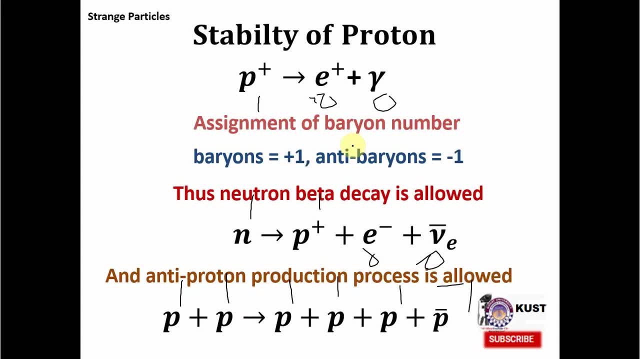 So far, so good. We have discovered another conservation law, that is, conservation of baryon numbers, and we have now a new baryon other than proton and neutron, a new baryon which is called a lambda particle, And again, this was not restricted here. 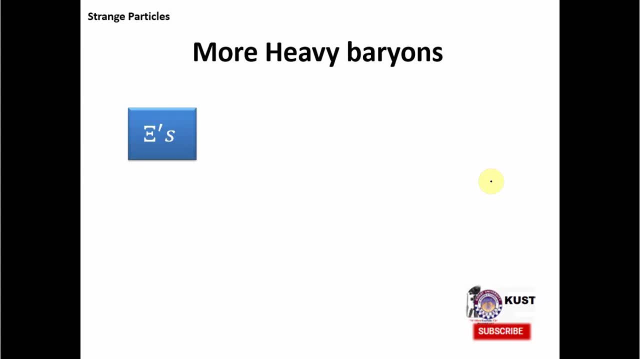 and we got few, not few, but few more other lambdas sigmas, lambdas omegas, and the list was extended into the hundreds of the particles. Actually, it is saying from Willius Lamy in his Nobel lecture: 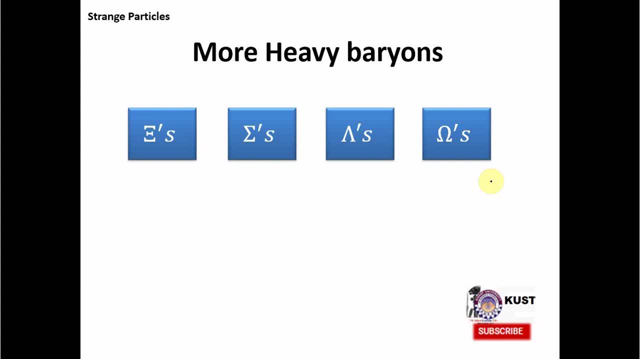 that in the beginning of the particle physics every new particle would win you a Nobel Prize. but later on there were so many particles discovered that now the discovery of another new particle ought to be punished by $10,000. And that was not fine, because that was complicating the picture. 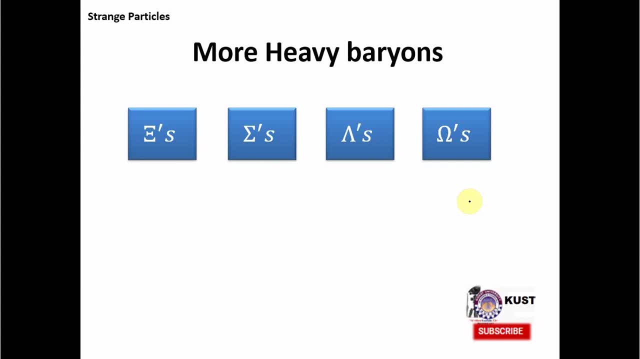 and physicists at that time were really in trouble in order to characterize these particles, in order to put them into the real places and understand their properties. But let's come back to this. so many particles, so many mesons and baryons discovered at that time. 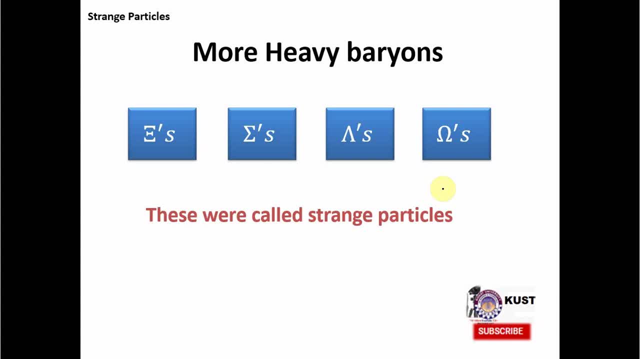 so that scientists were forced to call them strange, strange particles. So all these heavy baryons were called strange particles. But this is not only the reason that there are so many of them. there is another technical reason to call them strange particles. 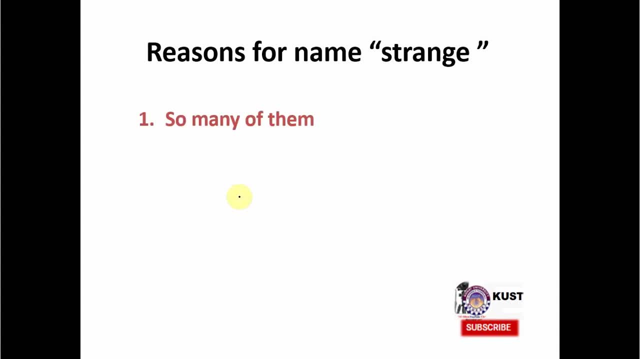 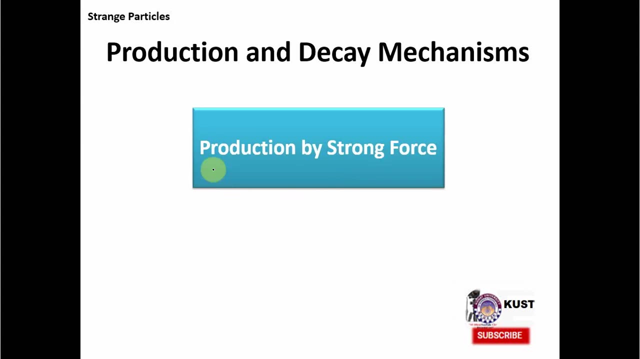 and this technical reason is the first reason is that so many of them? and this technical reason is that their production and decay mechanisms are completely different, and how they are different. Actually, these heavy baryons are produced by the mechanisms, by the mechanism of strong force, but they decay by weak force. 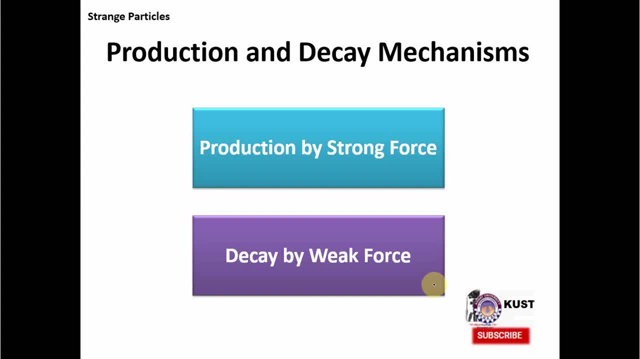 and that's really strange that a particle is produced by one force. these are two completely forces: strong force and weak force. they are produced by one force and decay by another force. This does not happen for other usual known particles at that time. 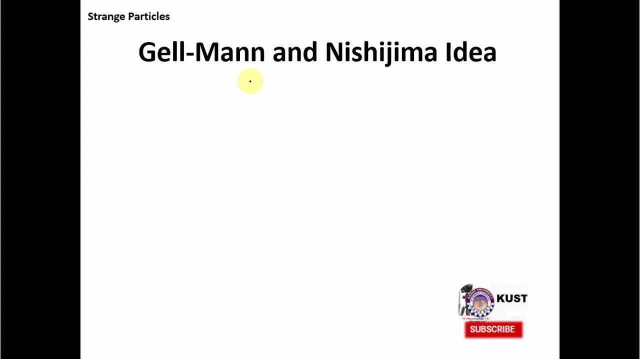 That's why Gelman, which is known as the Mendeleev of particle physics in Nishima at that time gave the idea of strangeness, and they said that in 1953 Gelman and Nishima suggested a new property called strangeness. 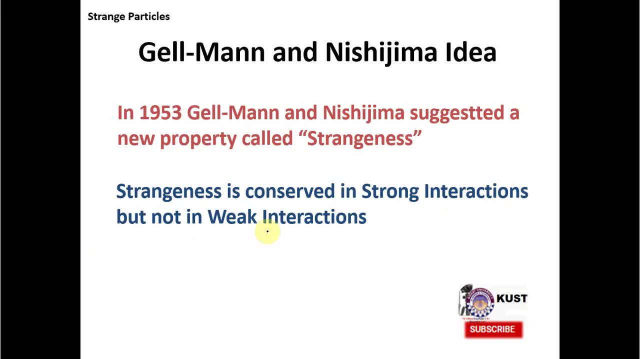 and strangeness is conserved in strong interactions, but not in weak interactions. That's why it is called strange. At that time it looked very strange, although there are so many other things which are strange, but Gelman had an idea to call them strange. 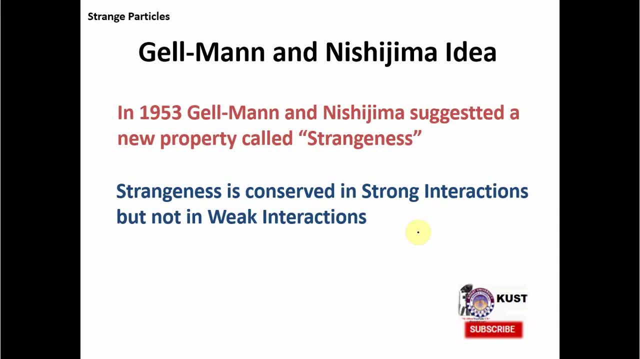 and they actually quantified this strangeness and given it a quantum number which can measure the strangeness of a particle. So now we know that these strange heavy baryons are actually strange because there were so many of them at that time. 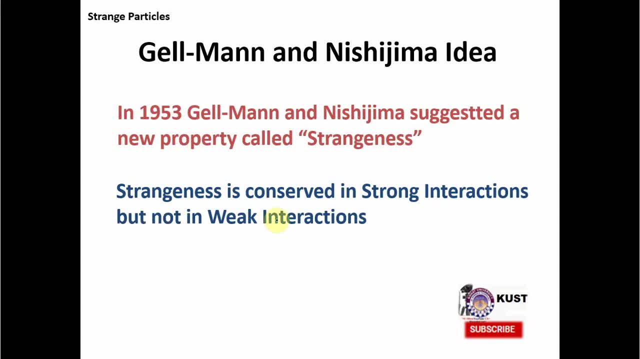 and also because the strangeness is not conserved in strong interactions. conserved in strong interactions, but not conserved in weak interactions. So the decay mechanism and the production mechanism are completely different. Now let's at the end of this lecture 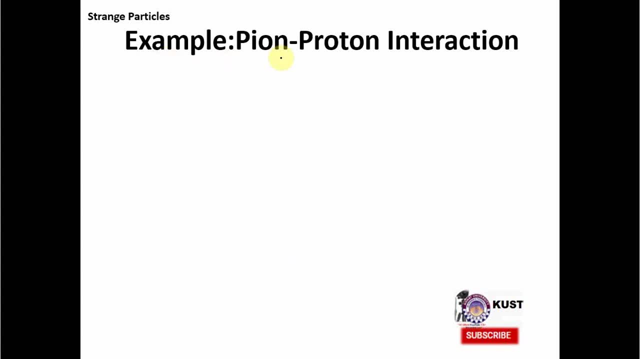 go into one concrete example of baryon-proton interaction and see that how strangeness is conserved into the one decay into the production mode and not conserved into the decay mode. So if we produce two strange particles, for example in this interaction, you can see. 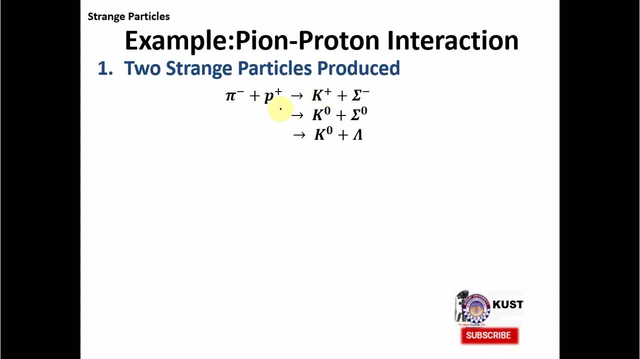 there are three possibilities that baryon and protons are actually collided and they can produce kaons, positive kaon and negative kaons, plus some other heavy baryons, If you assign strangeness, plus one here and minus one here and zero there. 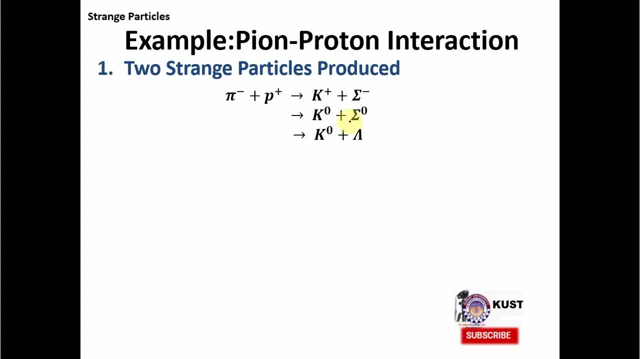 so you see that this in production, the strangeness is conserved. So zero here, because these baryon and proton have zero strangeness, Although this assignment of strangeness is completely arbitrary. but whatever mechanism you choose, you will find out. 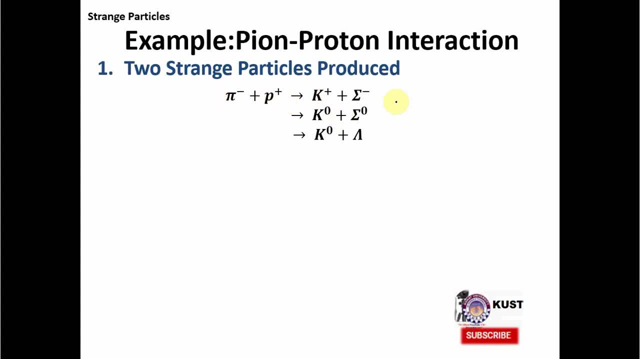 you will find out that strangeness is completely conserved here. So plus one minus one and zero zero here. So zero, total zero, here, total zero and all three of them. And you see that because of this conservation of strangeness, 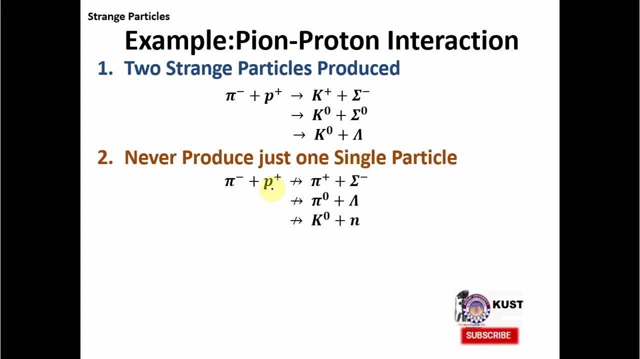 we never produced just a single particle. For example, these processes are not allowed because strangeness is zero here, but here is minus one, so this is not allowed, and so on. in this case, and this case, This strangeness is not conserved in the production mechanism.